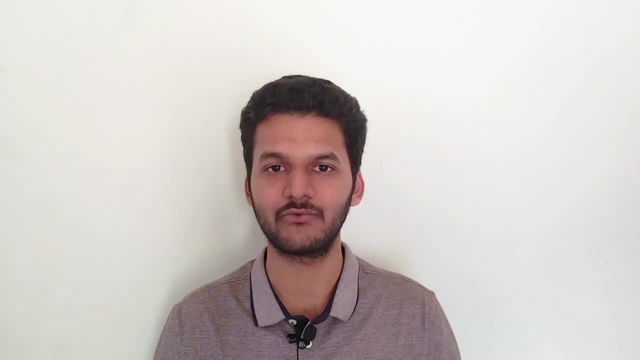 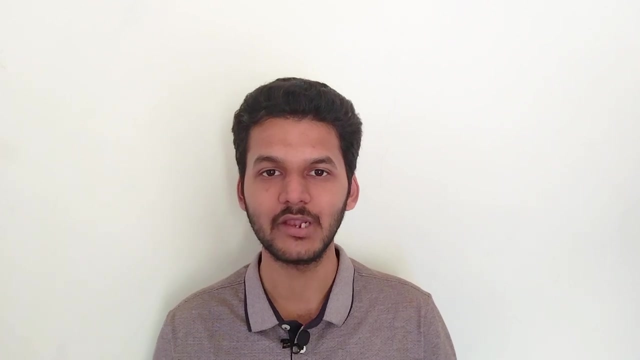 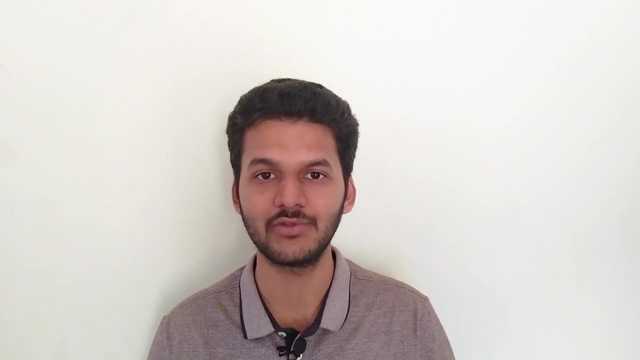 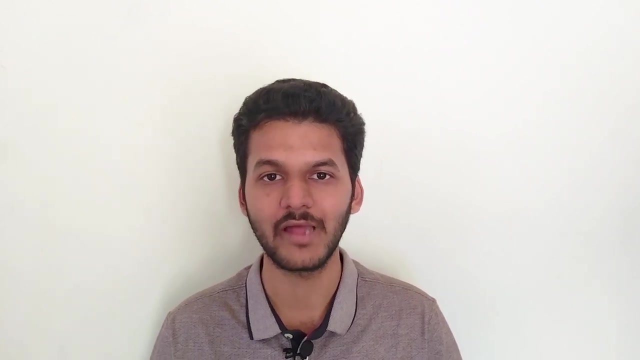 Now, what's important in robotics, Hardware or software? Both are important, Like software is also important, and the hardware as well, because both are interconnected. As any one of them is not present, it doesn't complete the system. Simplifying this further, we have electronics, design and coding. In the electronics part, we have microcontrollers, microprocessors, That is, the brain of the robot, the driving system, the controllers and sensors, actuators, all those things. We will focus on that part in this series. For design, we will be using Fusion 360.. 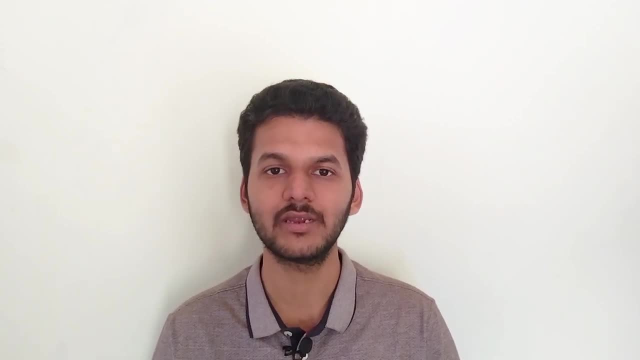 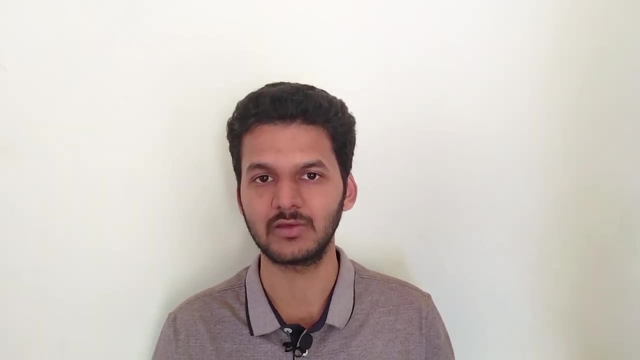 We will be using Fusion 360 software, which is a good way to convert the model into URDF, because the conversion process is quite easy as compared to other softwares like SOLIDWORKS and also you get very less errors while the conversion. For coding, we will be using Python, because Python is very easy to use for beginners as well as for the intermediate people in robotics. It also gives a variety of libraries, because we will be also focusing on the computer and the software. So we will be using Python because Python is very easy to use for beginners as well as for the intermediate people in robotics. For coding. we will be using Python, because Python is very easy to use for beginners as well as for the intermediate people in robotics. It also gives a variety of libraries, because Python is very easy to use for beginners as well as for the intermediate people in robotics. For coding. we will be using Python, because Python is very easy to use for beginners as well as for the intermediate people in robotics. It also gives a variety of libraries, because Python is very easy to use for beginners as well as for the intermediate people in robotics. For coding we will be using Python, because Python is very easy to use for beginners as well as for the intermediate people in robotics. For coding, we will be using Python because Python is very easy to use for beginners as well as for the intermediate people in robotics. 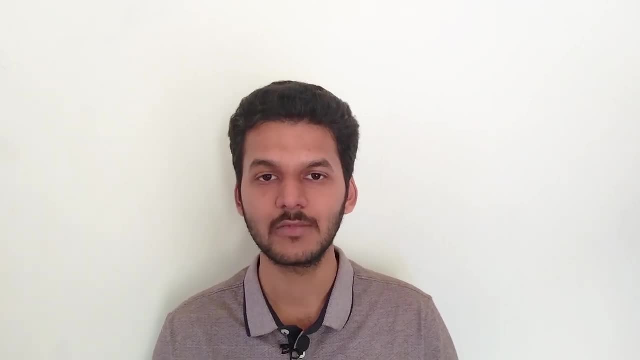 For coding. we will be using Python, because Python is very easy to use for beginners as well as for the intermediate people in robotics, so you can check it out as well. so this was for day one. we have only covered the basics of robotics, like what we will be doing in the 50 days, or else what is robotics? we will move very slowly. 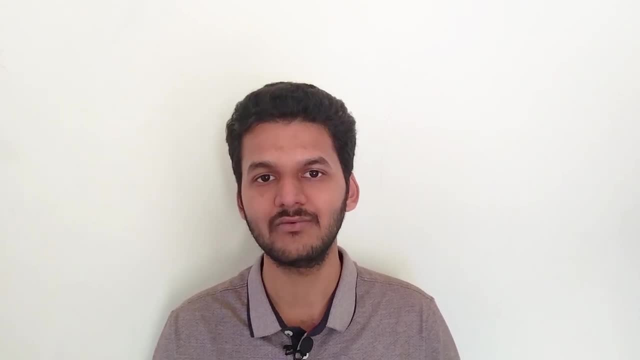 because we have to cover the basics and then slightly we will increase the level. with ROS as well. we will try to cover ROS 1 and ROS 2. the things we discussed are also available online so you can do a research on that as well. i will share the resources with you on the community. 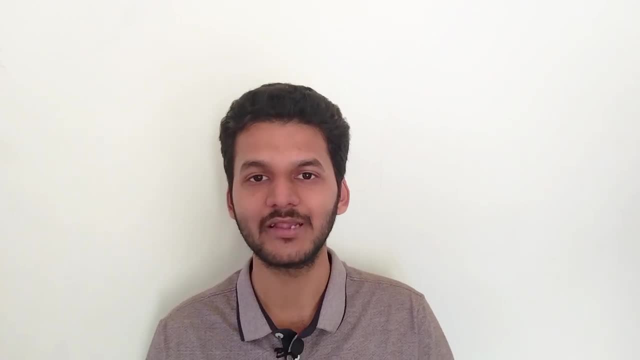 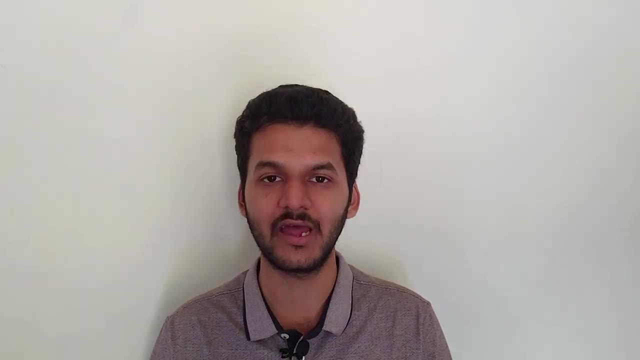 the projects will be on both simulation and hardware and the topics will be released soon. also, if you are following this challenge, you can use the hashtag 50 days of robotics and post that on linkedin, and there might be a delay in posting the videos on youtube.